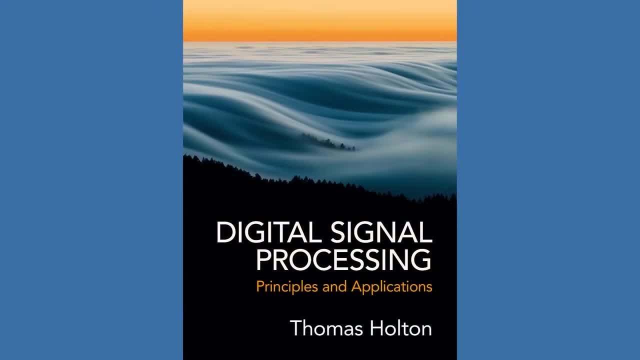 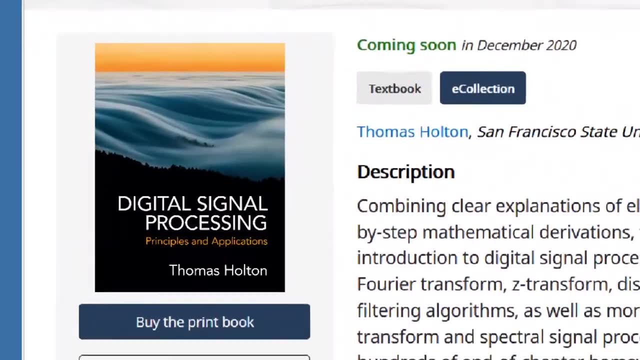 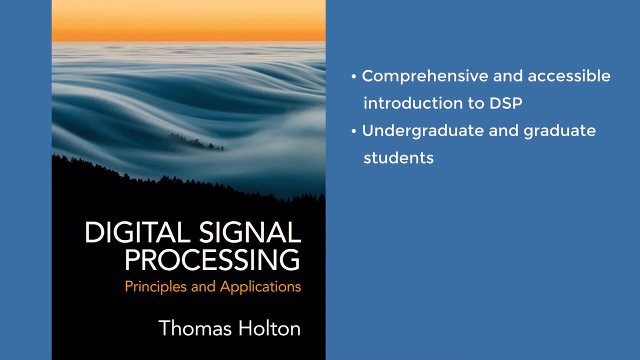 Hi, this is Tom Holton. I'd like to share with you some features of my new DSP book, which has just been published by Cambridge University Press. This book is designed to provide a comprehensive yet accessible introduction to DSP for students with a range of mathematical skills. The book starts with patient. 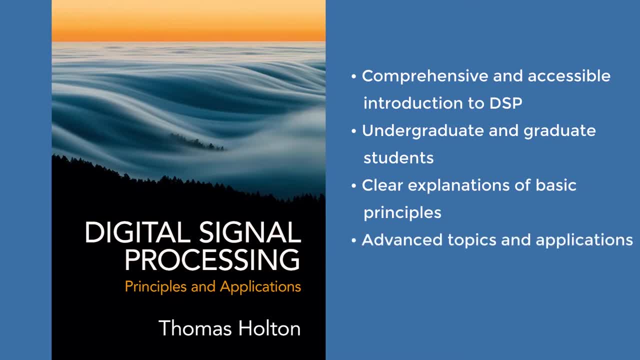 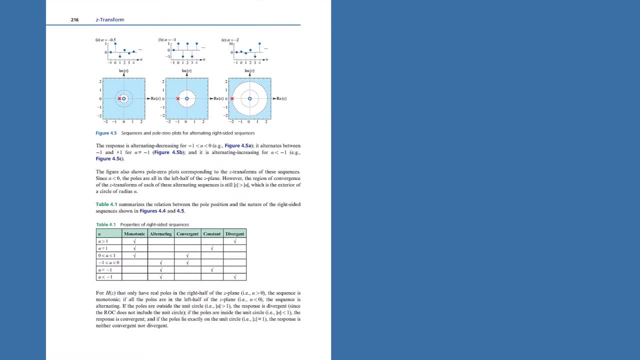 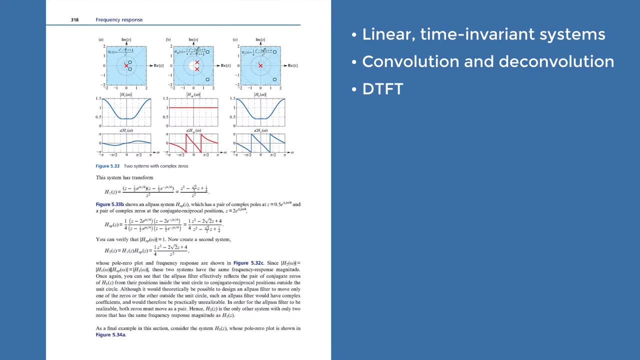 clear explanations of elementary principles and then proceeds to more advanced topics and applications. All the key elementary topics are covered first, including the basics of linear time, invariant systems, convolution and deconvolution, discrete time, Fourier transform, Z-transform, A-to-D and D-to-A conversion, including a discussion of hardware. 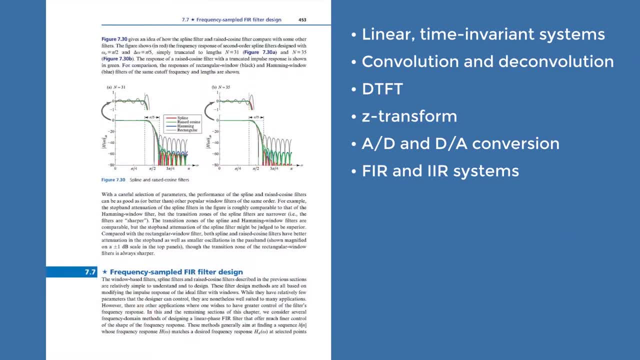 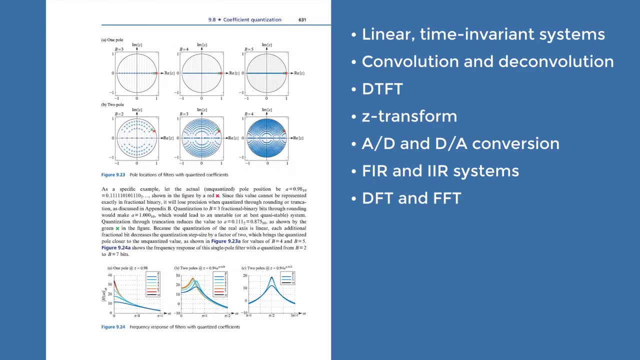 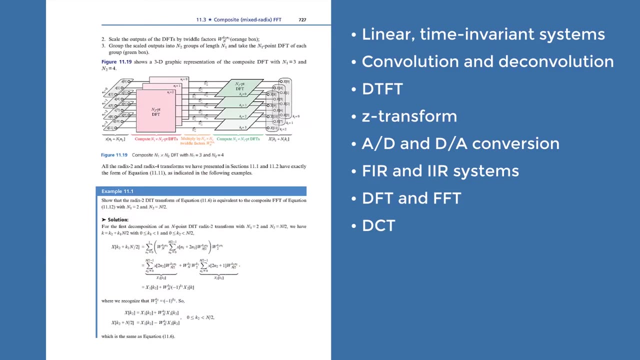 an extensive treatment of both finite impulse response and infinite impulse response, filtering algorithms and architecture, the discrete Fourier transform and the FFT. The later chapters of the book include a selection of more advanced topics, such as the discrete cosine transform and its applications, multirate and polyphase systems. 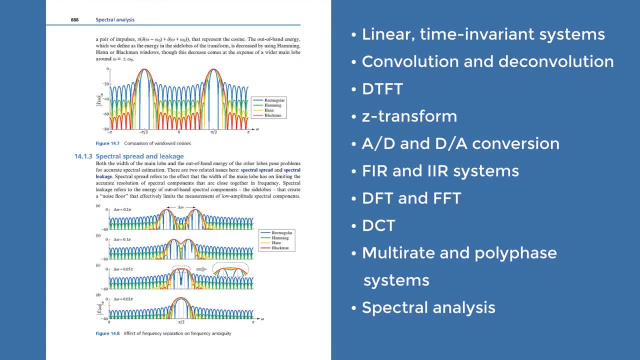 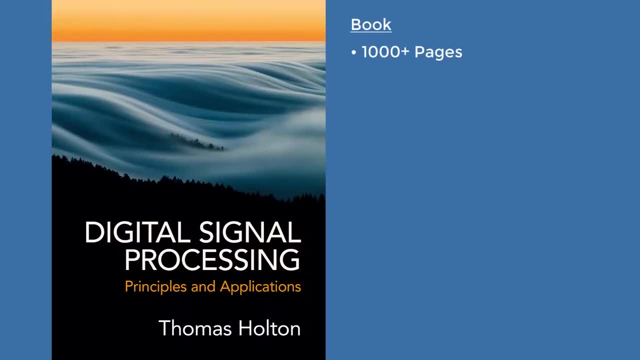 and a selection of topics in spectral analysis, including both parametric and nonparametric methods of spectral estimation. The book contains over a thousand pages, more than 600 full-color illustrations, 200 fully worked examples, hundreds of end-of-chapter homework problems and many detailed computational examples and applications. 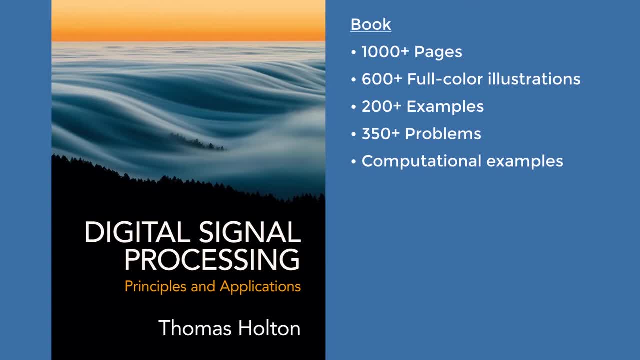 implemented from scratch in MATLAB. An extensive collection of supplementary material accompanies the book online, including over a hundred pages of text with 70 illustrations covering advanced topics such as the MDCT and filter banks. There's a full set of solutions and a selection of MATLAB exercises for students. Finally, for instructors, I have something special. 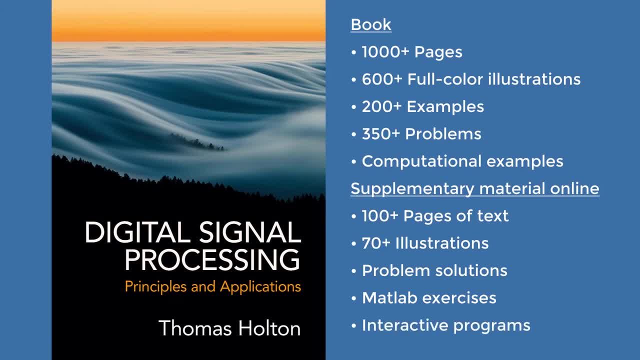 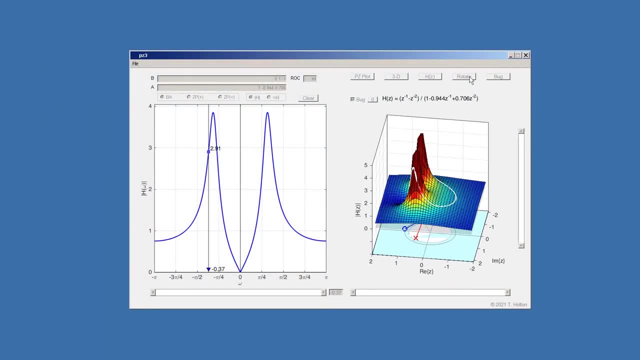 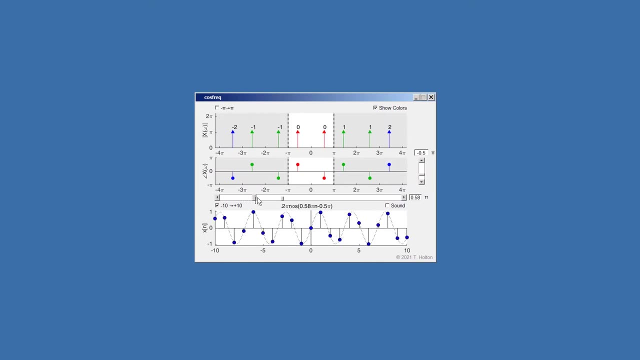 Over the years, I have developed a suite of interactive programs to help explain DSP concepts to my students during lectures. There are now well over two dozen programs covering many aspects of the material in the book, including complex exponentials and sinusoids, convolution, the DTFT. 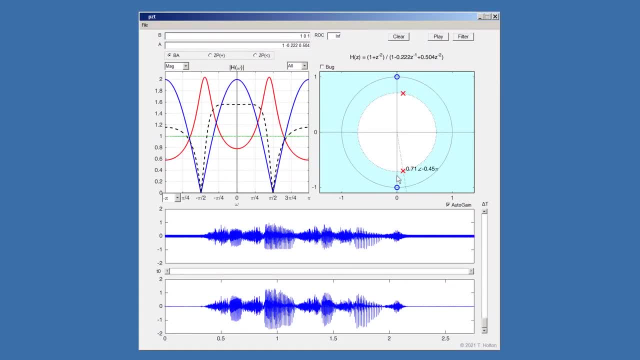 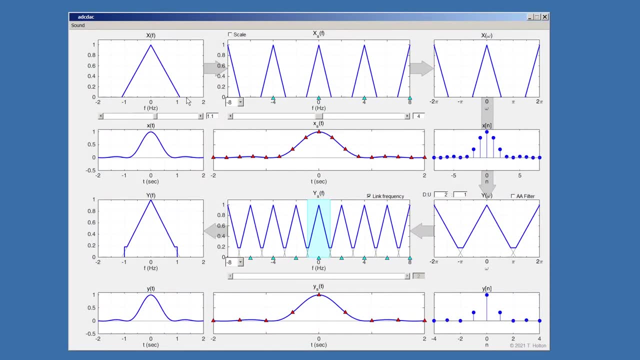 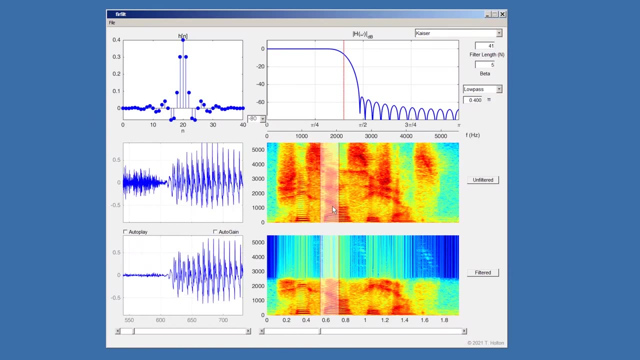 pole zero plots and their relation to frequency and impulse response A to D and D to A. conversion including upsampling, downsampling, resampling and aliasing. the design of many types of FIR filters and their application to the filtering of speech and other signals. the design of IIR.